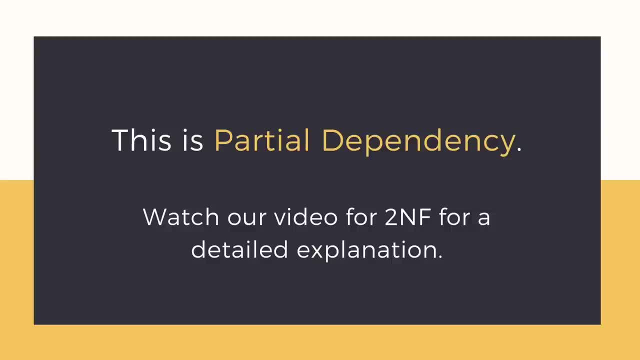 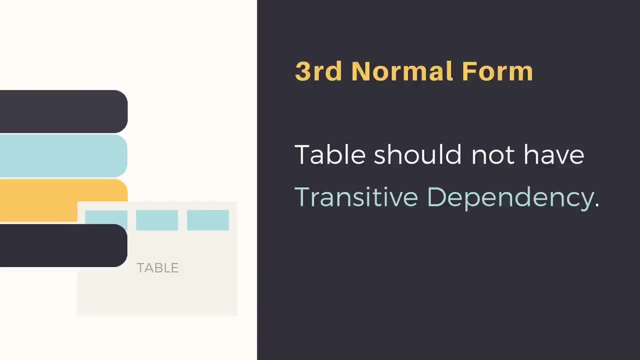 To learn about the concept in details, watch our video for the second normal form. For a table to be in the third normal form, it should be in the second normal form and there should be no transitive dependency, which means for a functional dependency, a derives b. 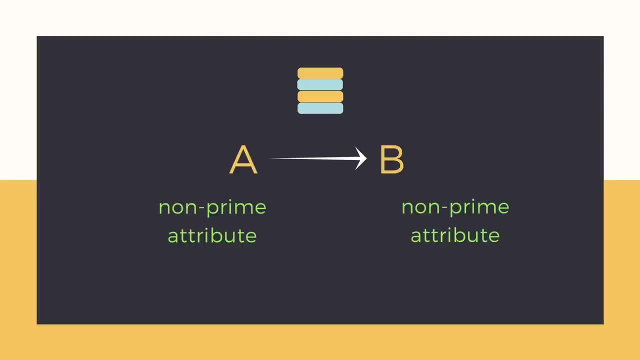 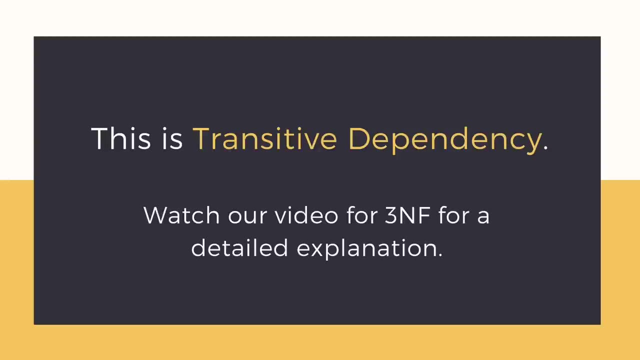 If a is non-prime and b is also non-prime, then this is known as transitive dependency, And to learn about this in detail, along with a simple example, go watch our video. for the third normal form, Now comes BCNF. For a table to be in BCNF, it must satisfy two conditions. 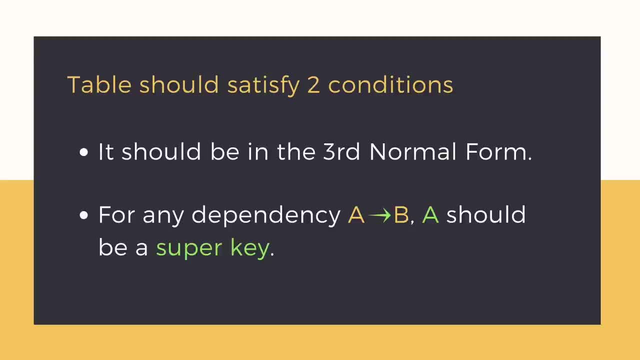 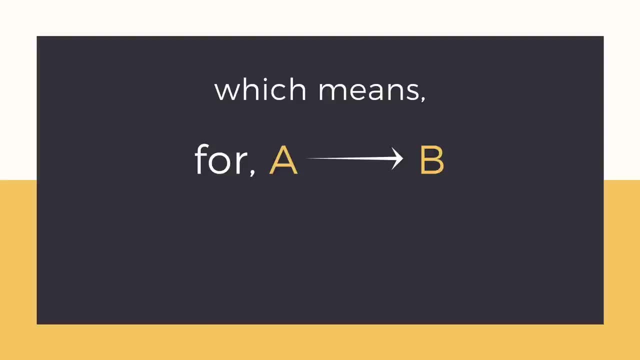 The table should be in the third normal form and for any dependency, a derives b. a should be a super key or in simple words, we can say: a cannot be non-prime attribute with b being a prime attribute. Until now we have seen non-prime attributes depend upon prime attributes. 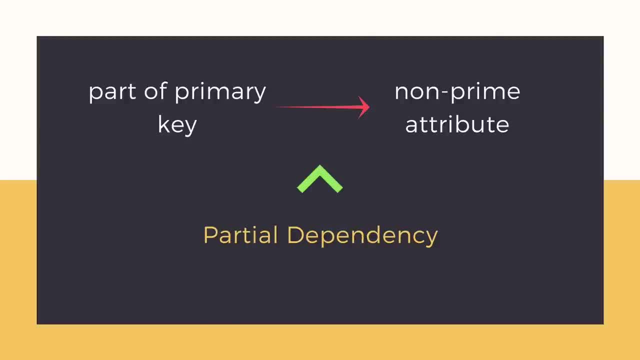 or a part of it, like in partial dependency, or some other non-prime attributes, like in transitive dependency. But what if a non-prime attribute depends on a non-prime attribute, A non-prime attribute starts deriving a prime attribute. BCNF doesn't allow this behavior. 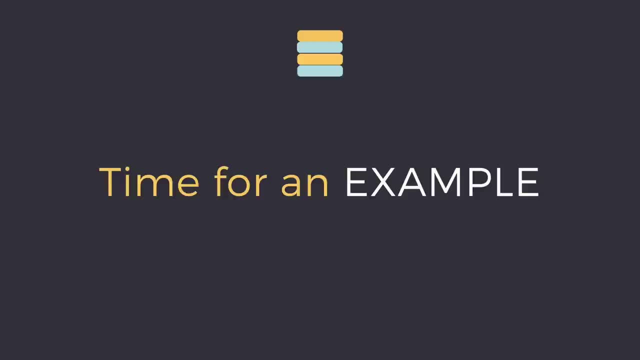 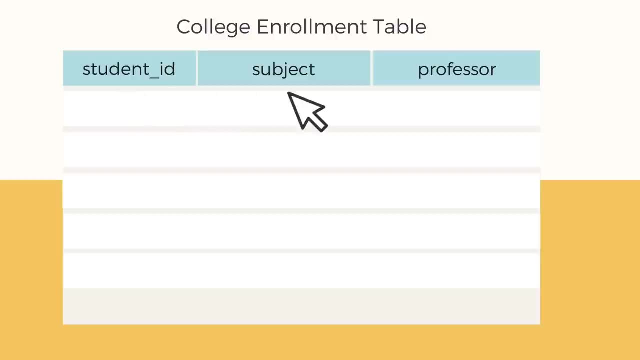 So let's take an example and try to understand this type of dependency. So we have a college enrollment table here where we save student id, subject opted by the student and the name of the professor assigned for that particular student for a particular subject. Let's add some data to our table. As you can see, now one student can enroll for multiple subjects. 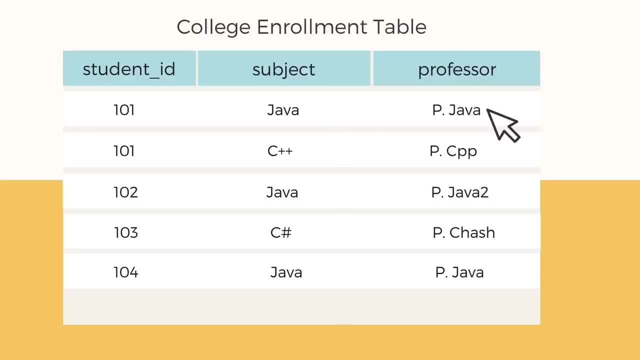 And for each subject a professor is assigned to the student. One important point to note here is that there can be multiple professors teaching one subject, like we have for java, pjava and pjava2.. In this table, the student id and subject together form the primary key, because we can use student id and subject together to find 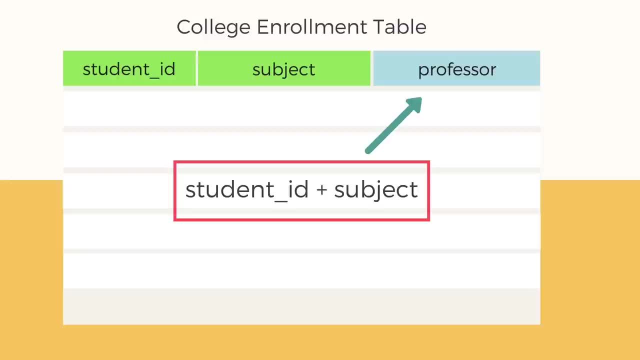 all the other table columns. Well, in our case there is just one another column. Also, as one professor teaches only one subject, we can use the professor column to find the subject name as well. Now, this table is in first normal form, as all the values are atomic columns have.